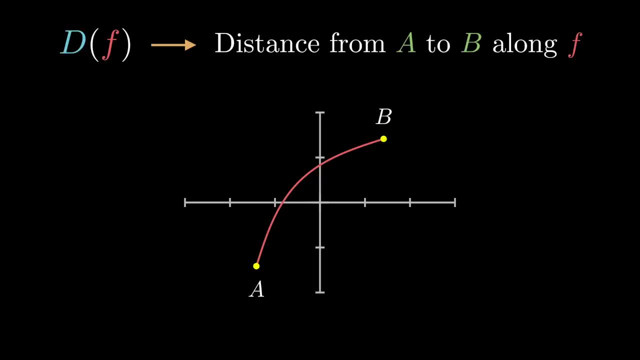 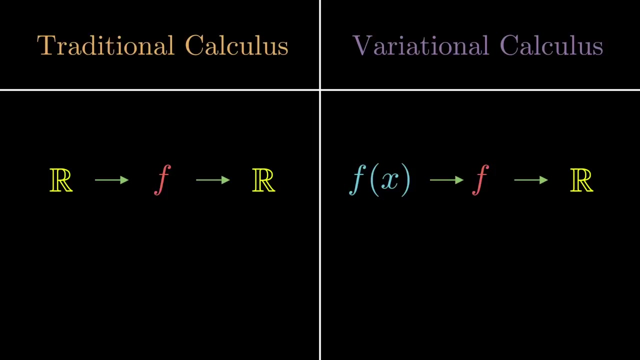 f. Variational calculus deals with finding stationary points of these functionals. Notice the difference: In the traditional calculus case we have a function that maps from real to real, But in the variational calculus case we have a function that maps from function to real. In both cases we're finding stationary states of the function. 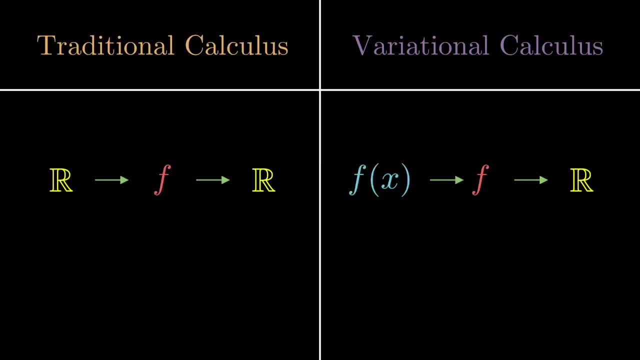 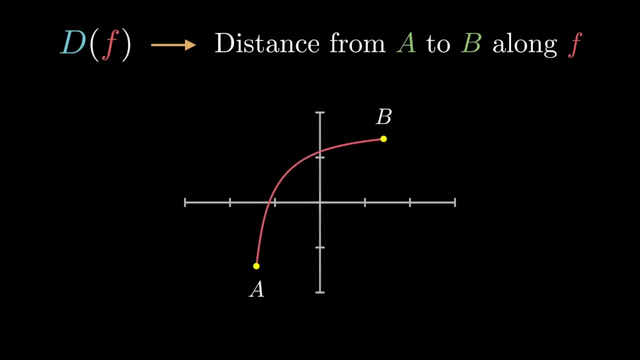 but traditional calculus tries to find a stationary point where variational calculus tries to find a stationary function. Let's consider the distance example again. Given two points, a and b, the distance functional takes in some function f And outputs the distance along that function between a and b. 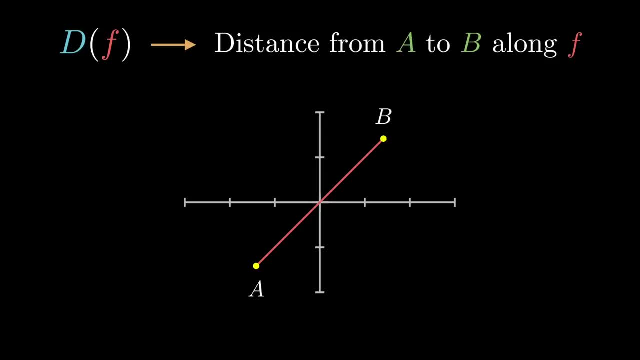 Now, the goal is to minimize this distance functional. Now, obviously, the function that minimizes this distance functional is a straight line. But let's look at what this distance functional would look like. Considering points a and b have x, coordinates, x1 and x2, the distance functional can be. 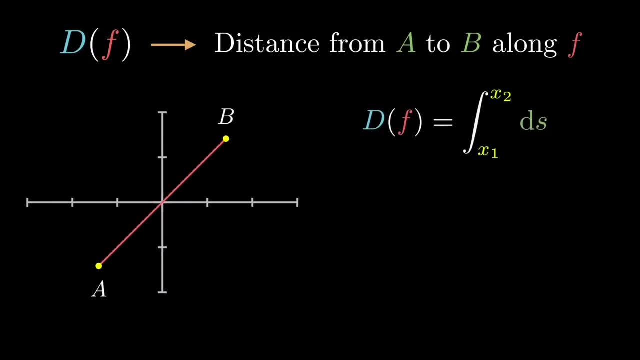 written as the arc length from x1 to x2 along f. Using the formula of arc length from calculus 2, we can write this distance functional. If we reframe the problem, we can say that the goal is to find some function f that minimizes. 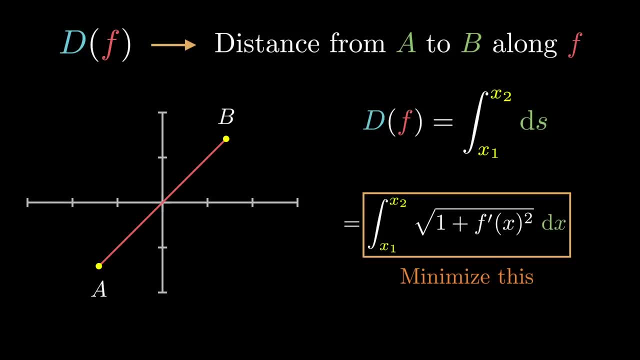 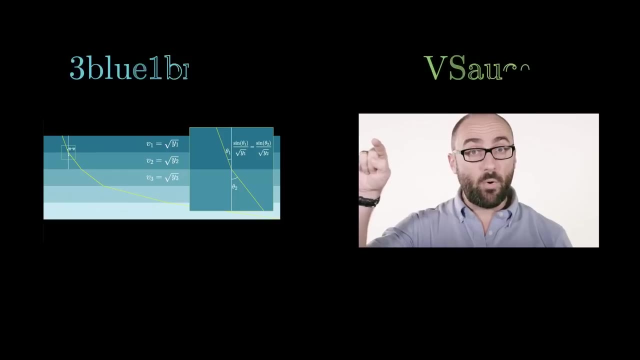 this integral. This example can get more and more complicated. What if, as we move along the path, we are obstructed by friction that changes the velocity? What if there's gravity? In the case of gravity, this problem has a special name: the brocistochrone problem. You might have seen videos by Vsauce. 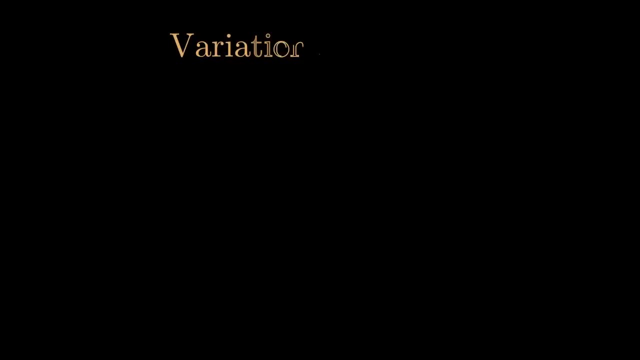 or 3blue1brown on this topic. A more general way to write the problem, variational calculus, is to find some function f such that the integral from x1 to x2, of capital F, of xf, of xf, prime of x is a stationary point. Notice, the integrand has a function that takes f. 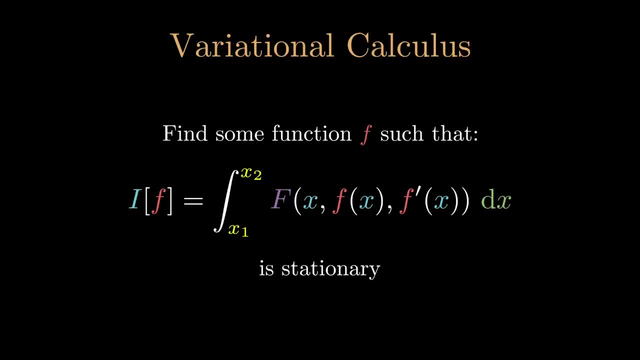 prime of x as an input. This is something we did in the distance functional too. This function, capital F, is called the Lagrangian. Now you may ask how do we solve this question? I'm going to pass it back to Papa Flamie, to. 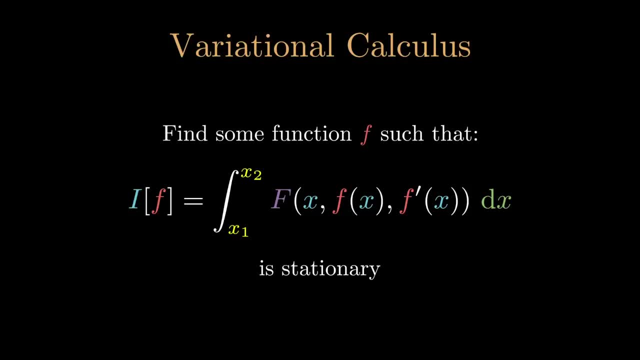 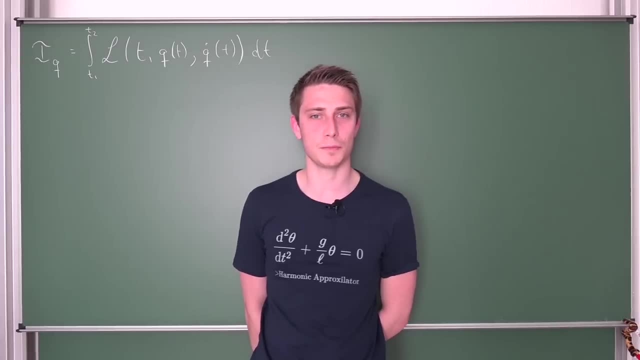 derive the Euler Lagrangian. Good morning, My name is Papa Flamie. if you don't know me, link probably down in the description. If you know me, hello from the papa to everyone out there. Thanks to vcubingx for having me. 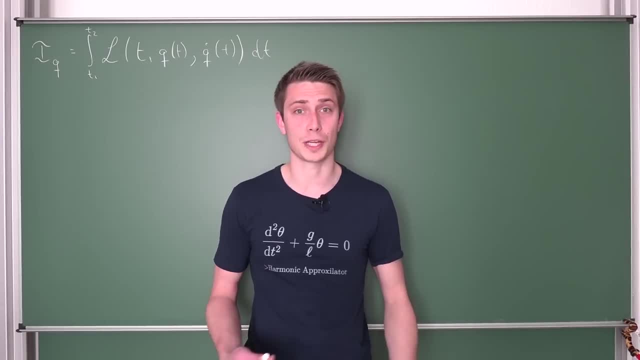 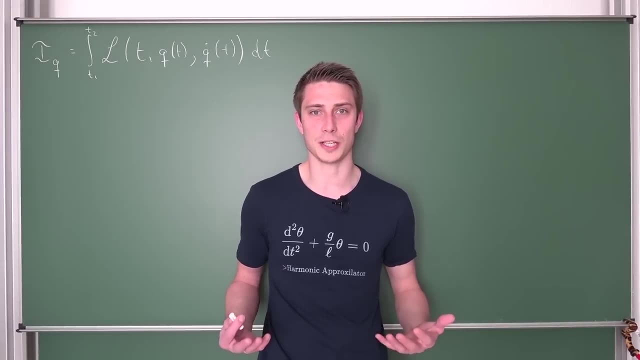 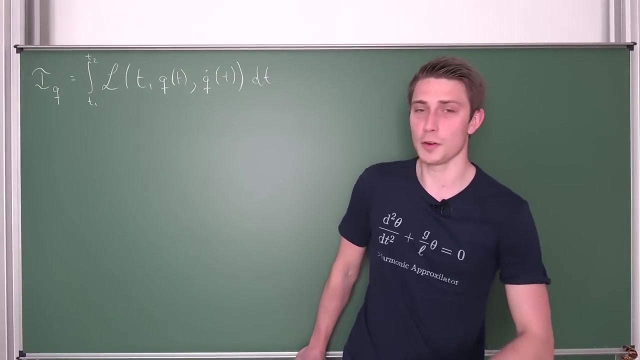 here on this show. He already did a little introductory part for the calculus of variations and now we would like to derive basically one of the most important partial differential equations there is in mathematics. So first I would like to start off by telling you what this right here is. This is what 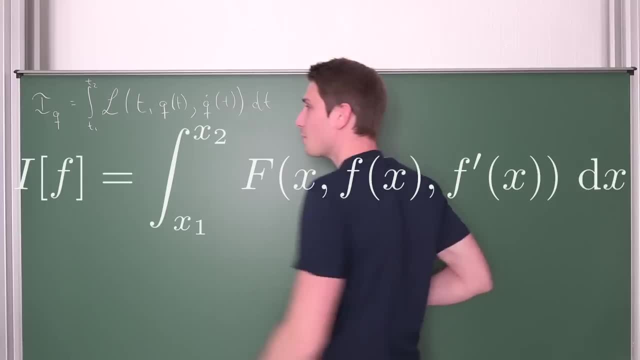 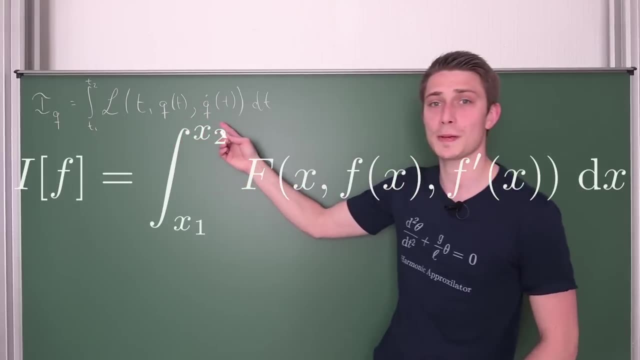 we had before, where vcubingx used capital F here and instead of q he used, for example, x. So I'm using 30 physicist notation. those are our constraints. basically, t is just the time and q dot is the time derivative of q. 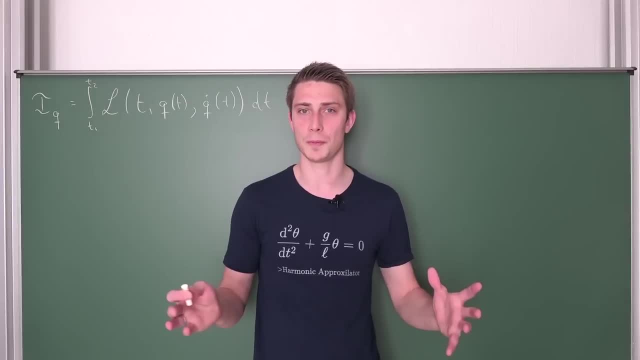 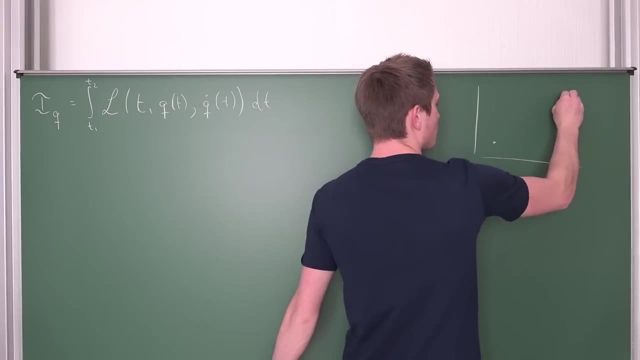 Now, with that out of the way, we would like to take a look at optimization, at minimizing a problem. for example, We are going to take a look at a certain curve at first. so let's say it goes from two nodes, so t1 to t2, and this is our curve, for example, 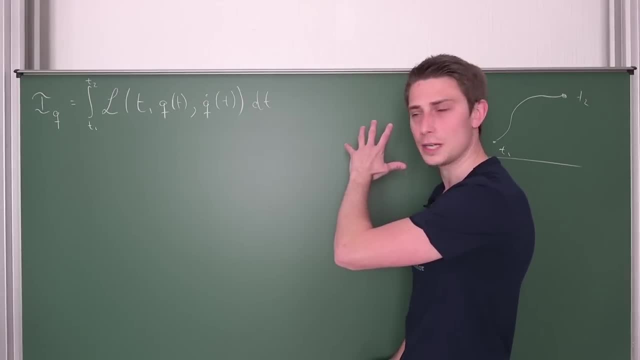 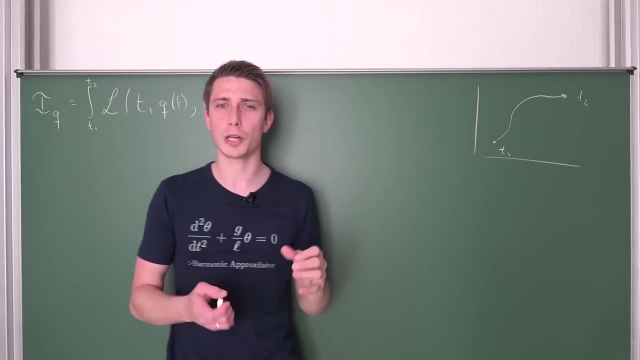 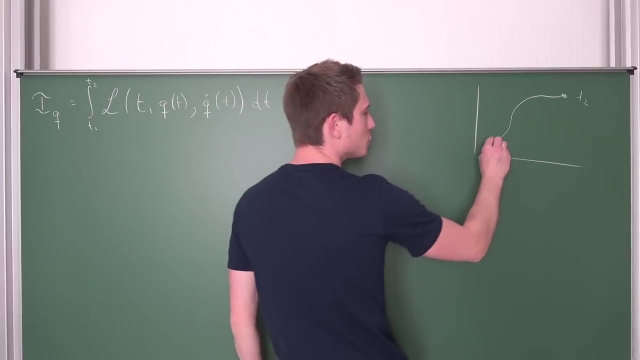 Now let us say that this curve is already optimized, So meaning q in here is going to minimize our function in some way. Now we would like to add a little bit of noise to this function. we would like to put a little bit of error in meaning. let's say, for example, we are going to choose nearly the same curve. 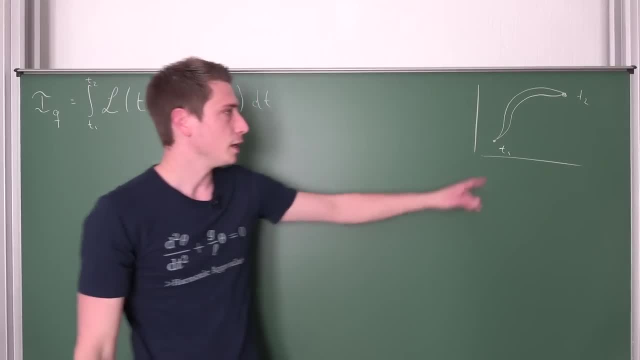 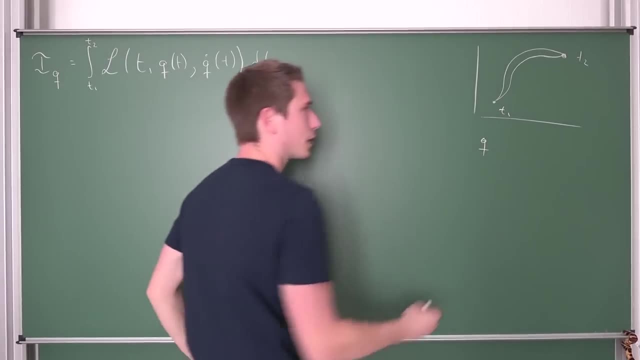 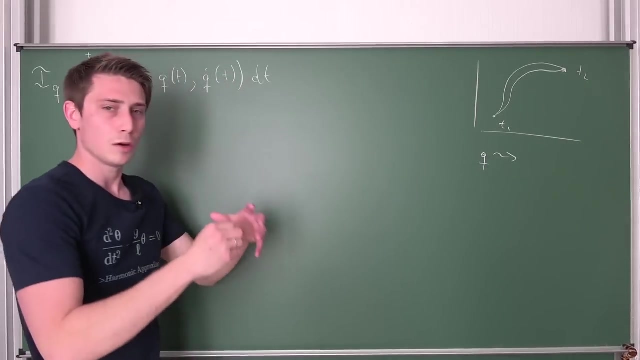 just a little bit stretched outwards, for example. Now we would like to describe this new path of this curve. We are going to do a little transformation. our original q- okay, it's the function between those two nodes, t1 and t2, is going to be transformed into. we are going to have our 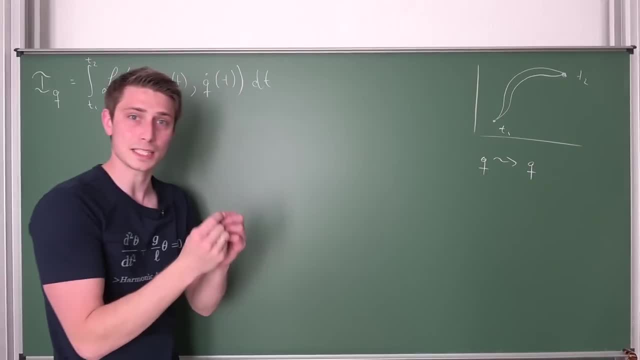 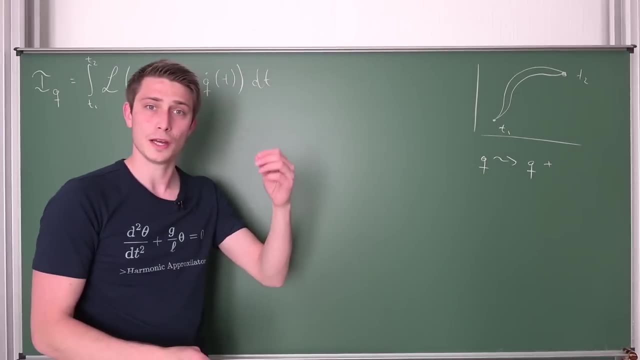 original path q, yet again, plus this arrow term that we are going to have. We are going to give it a certain notation, We are going to give it a certain path. Okay, The degree of variation is just a real number. it could also be zero. okay, let's call it. 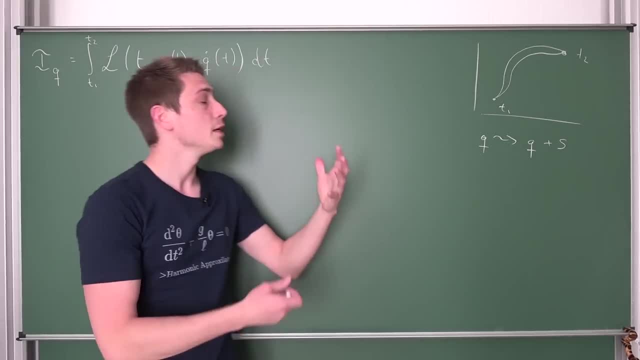 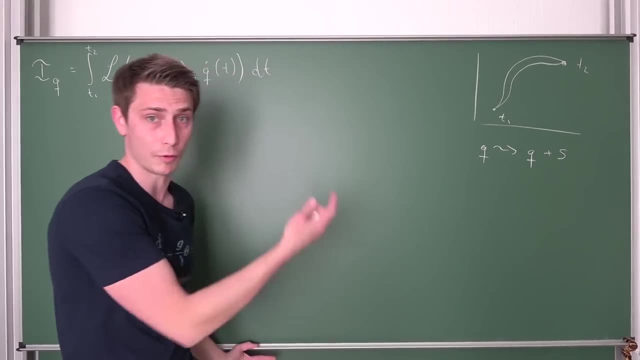 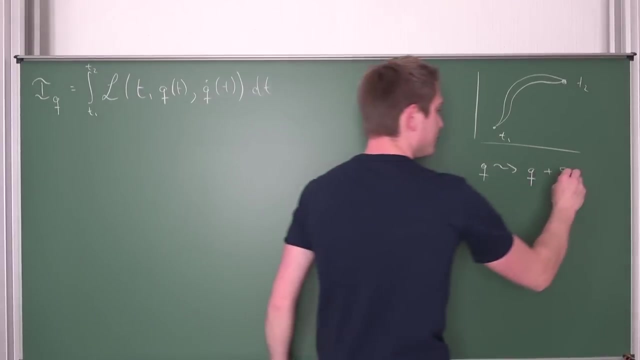 s. that's the degree of variation, And we would also like to put a little function on there, because you can only add functions of x basically together, or functions of t. That actually describes our stretching or our deformation of this path. This is the actual variation. we are going to call it delta q. 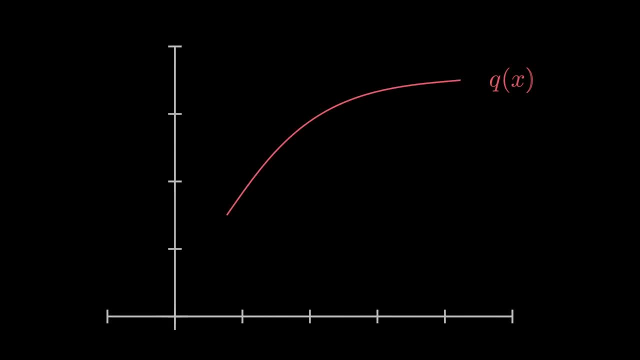 Before we move on, I just want to recap what happened When we calculated the derivative of a function. the way we did that was take a small step in the x direction and look at the resulting change in the y direction. This is basically the exact same thing. 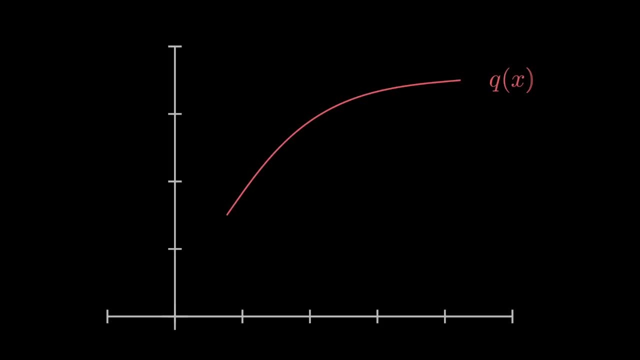 We have a functional and let's say the point we are looking at is q. So we take a small change in the functional, which is just a slightly different function. The change in the functional is another function, delta q, Since we want the endpoints of the similar function to be the same. the endpoints of 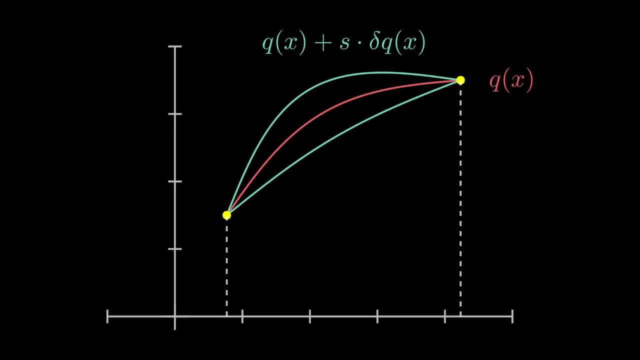 delta q at point t1 and t2 have to be the same, So we are going to take a small step in the x direction and look at the resulting change in the y direction. This is the exact same thing we did when we were taking the regular derivative. 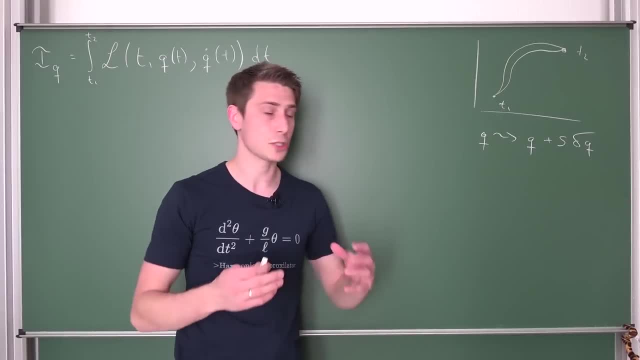 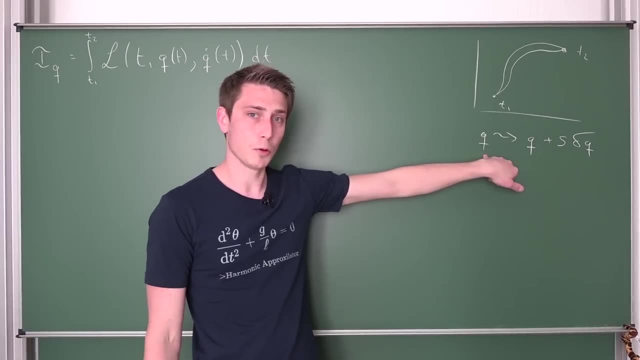 Now back to Jens to continue the proof. With that out of the way, I want you guys to notice something: Delta q is yet again a function with respect to t, And if we were to differentiate both sides here, this side and this side, we are going. 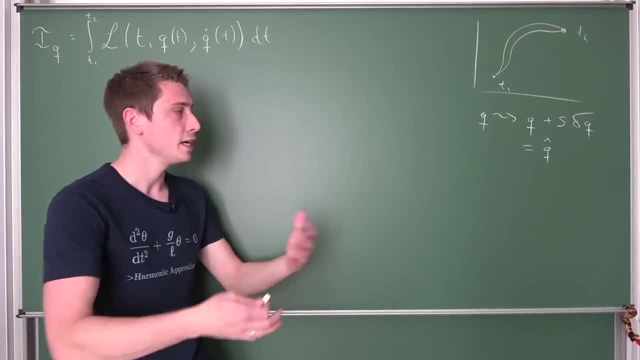 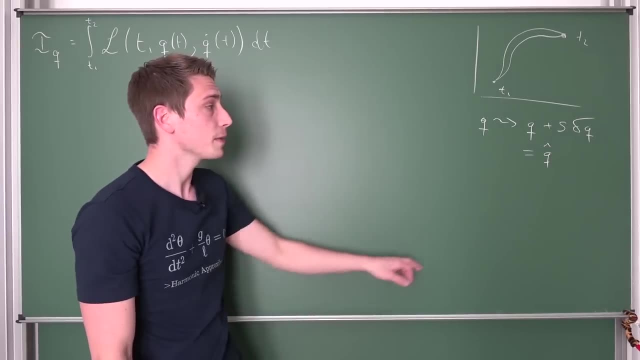 to give this thing a new name, q, For example. if you've ever done inverse problems, you might know that we are going to call a minimizer of a function head something x head. If we were to differentiate this thing with respect to time, this is just going to give. 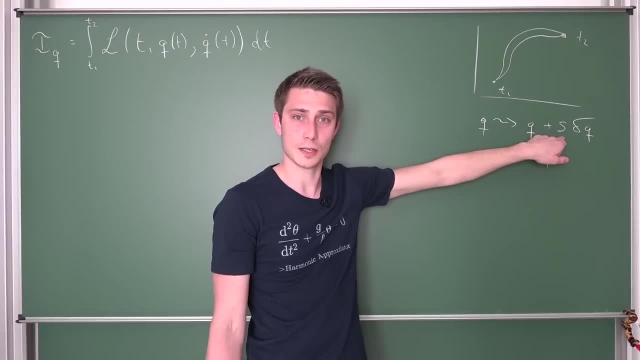 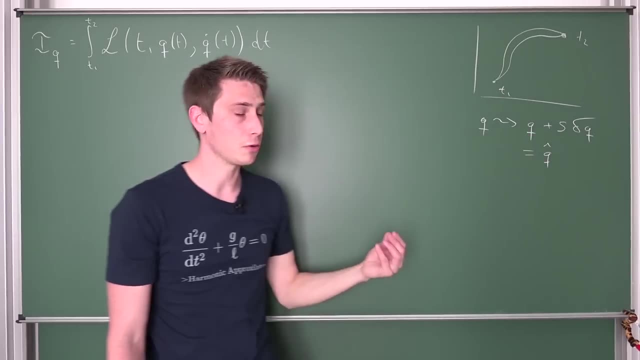 us q. And if we were to differentiate this left hand side here or this upper side, well, what are we going to get? This is just an additional thing. so we are going to use the linearity of the differential operator. meaning this is q, dot plus s. it's just a constant. it's going to stay where. 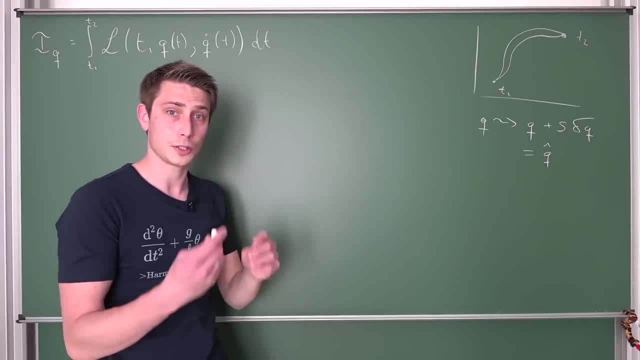 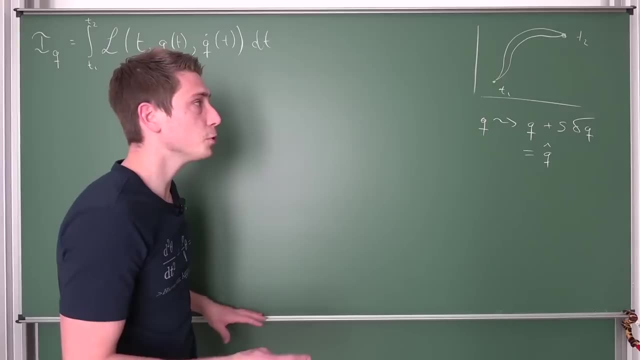 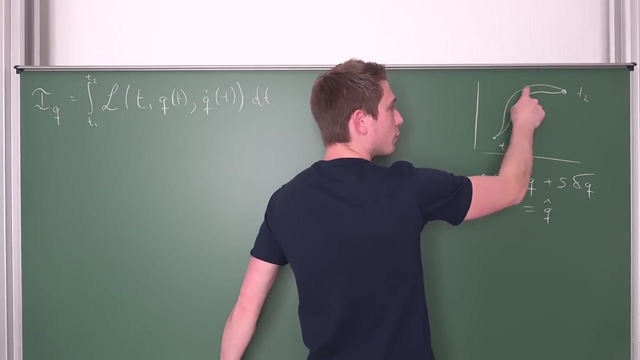 it is, and delta q dot, q dot plus s delta q dot. This is the differential of this thing. Okay, There was already some very important input. What other things could we say about this thing? Well, when would our Curve, our new curve, our new path, be equal to our old path? 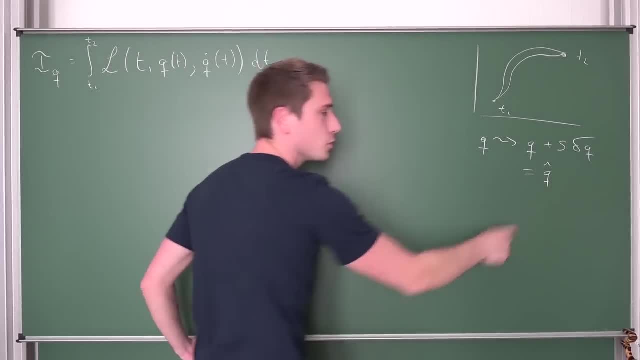 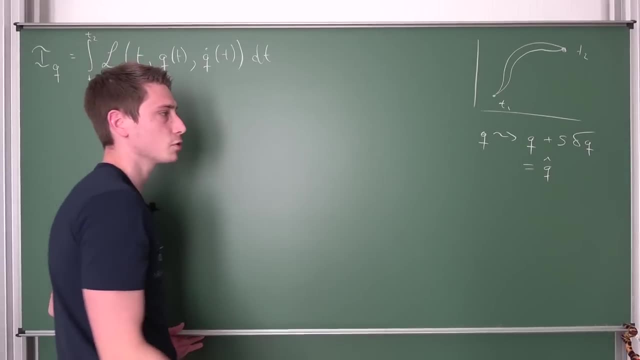 So here's the question: when is Q actually equal to our Q hat? When are we going to minimize this function exactly? Well, when our degree of variation is going to go to 0, so for s going to 0, we have the case that our Q hat. 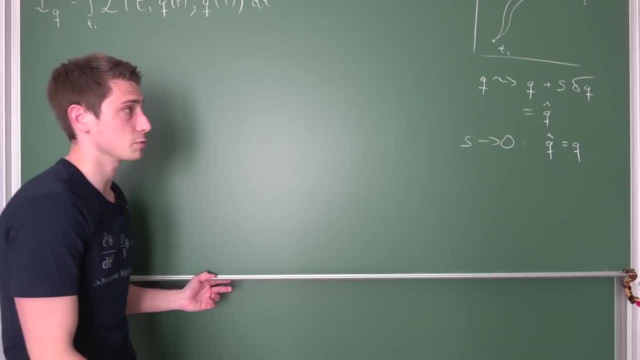 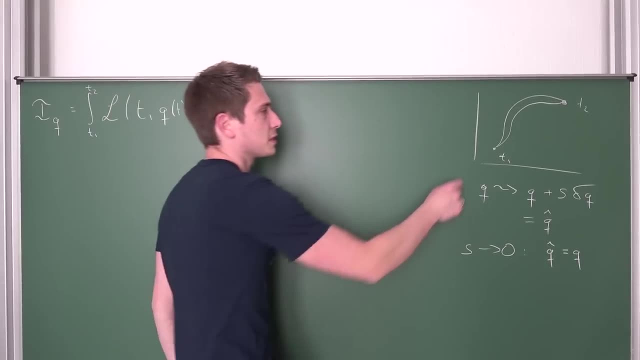 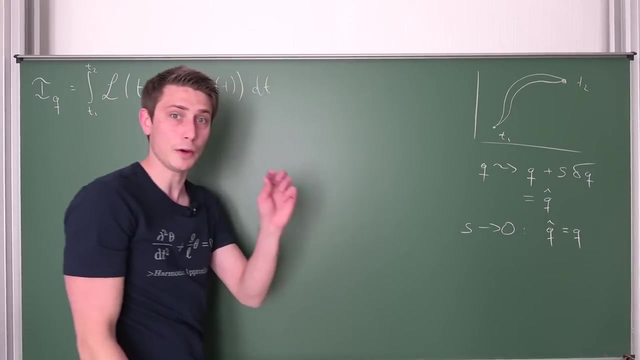 Is simply our Q. yet again, We are optimizing our curve this way, minimizing it in some way. Also, we would like to add some boundary conditions. I want you guys notice that the closer we get on this new path To our nodes, the closer it also gets to our original path that we have here. our arrow gets smaller and smaller, our variation. 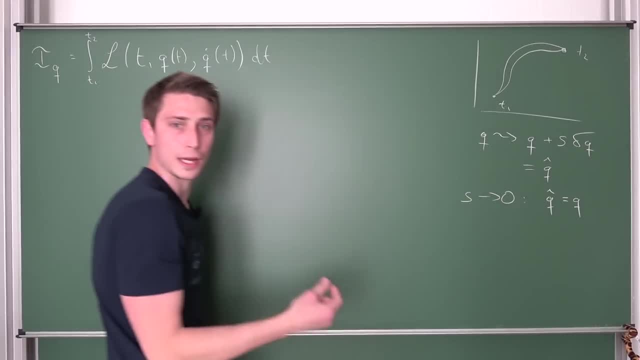 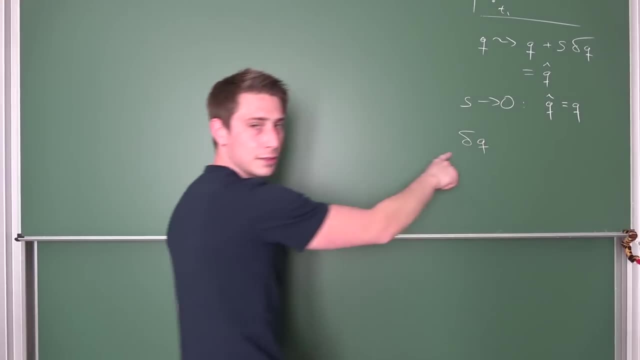 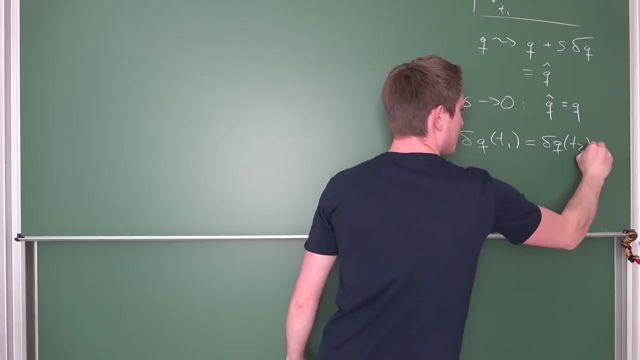 Becomes 0 there. this term, our arrow that we are have having our noise in this function is going to go to 0, So we are also going to have to condition That Q, our variation at the end points, Is actually equal to 0. okay, we do not have any variation anymore at our nodes. 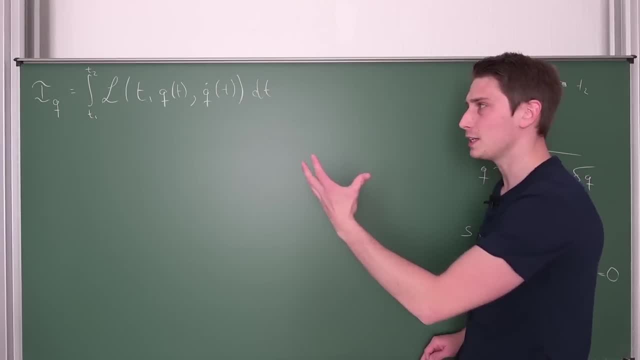 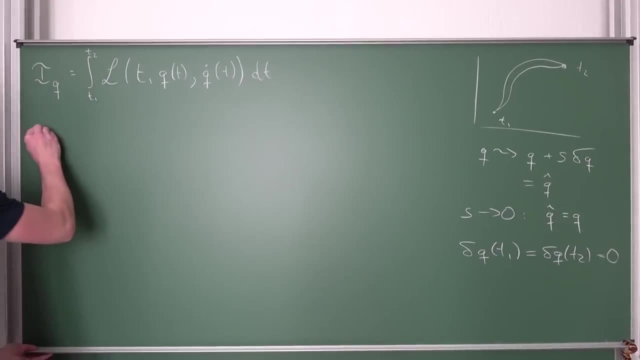 now All the basically hard work is already done And now we are going to do some playing around. We are going to do the transformation we did here on this integral meaning overall. We are going to do the transformation where Q goes to our variation path that we are having. 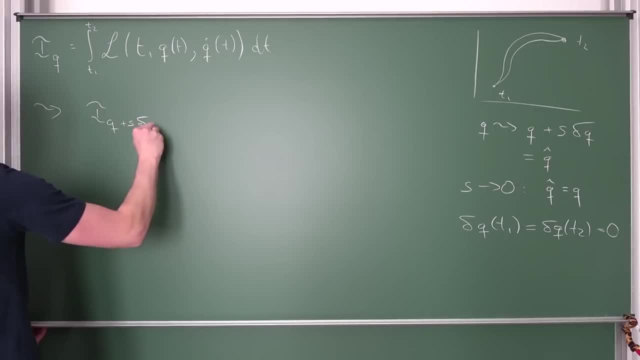 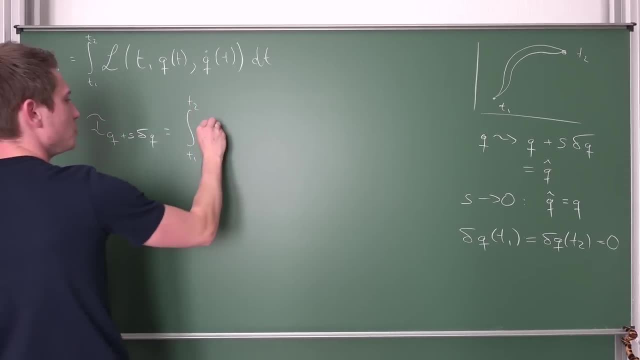 So I of Q plus s Delta Q is thus equal to well, all of this stuff plugged into here, Our path is still the same. integral from t1 to t2 of our Lagrangian. This is what you would call in physics a Lagrangian and then t comma. 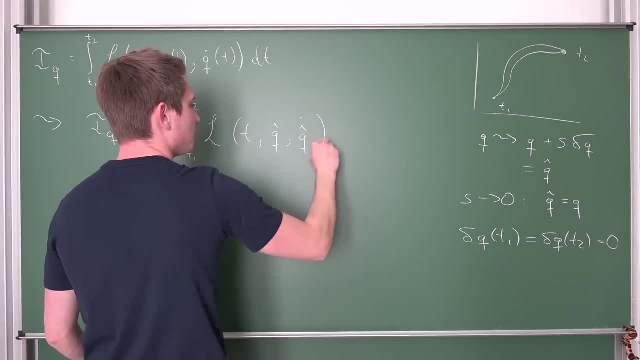 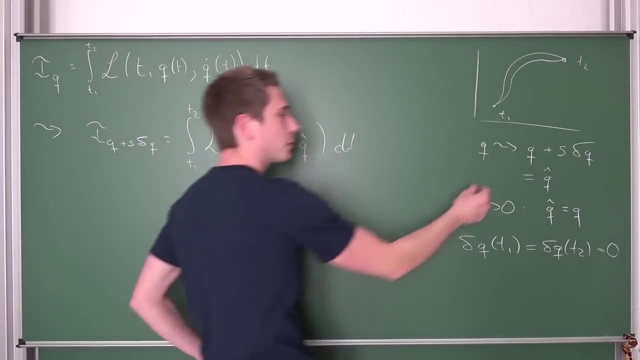 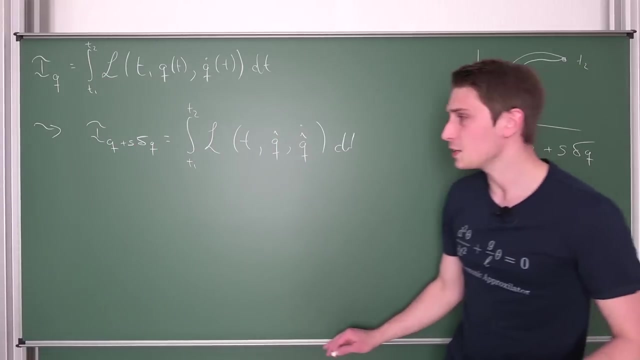 Q hat comma, Q hat dot. Like I said before, differentiating this thing is only like piecewise differentiation and that piecewise differentiation, but we are differentiating Each and every part in here. Okay, Now, this is what we have at the moment. Let us think again when our path is going to be minimized. if you take a look at regular calculus, 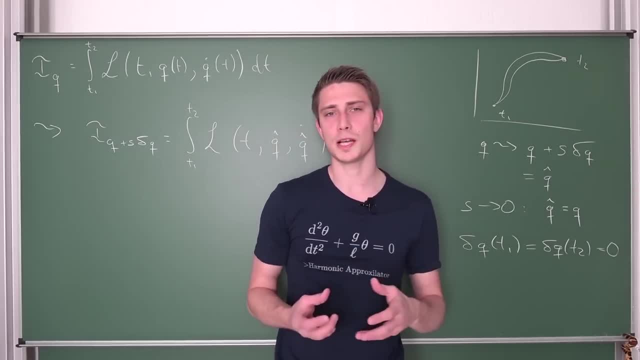 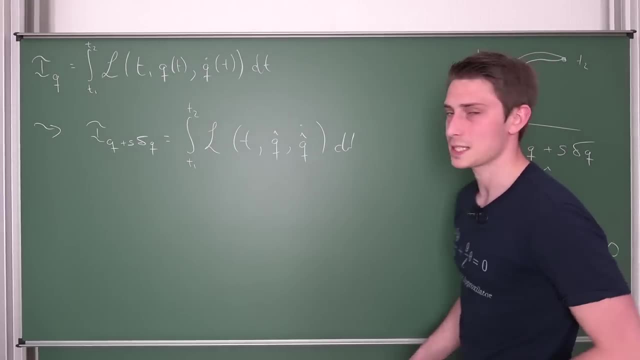 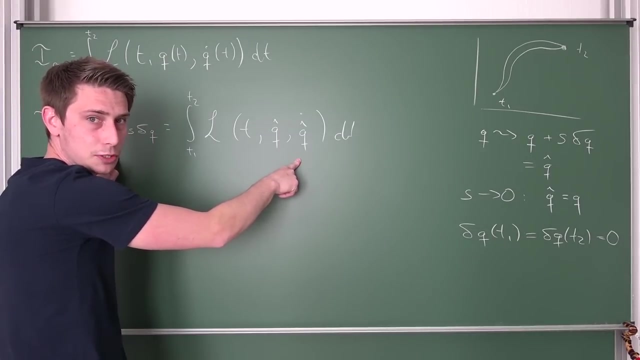 We know that if we take the first derivative of something and this is equal to 0, We know that there's a maximum or a minimum. in some way We are going to go by the same means here. We would like to differentiate this function and see when it's exactly equal to 0, okay. 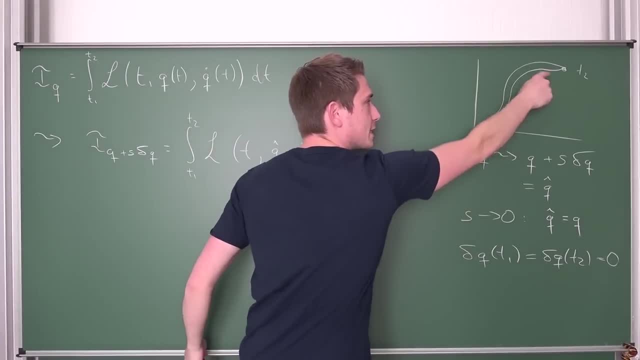 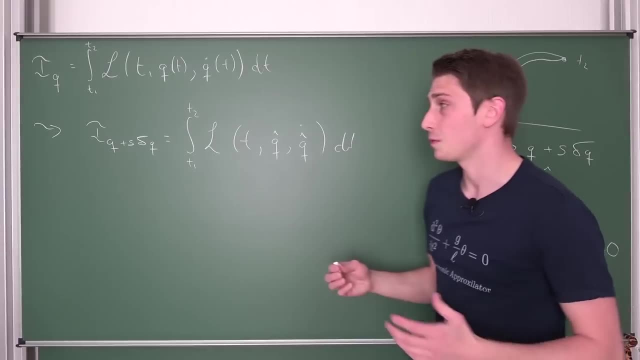 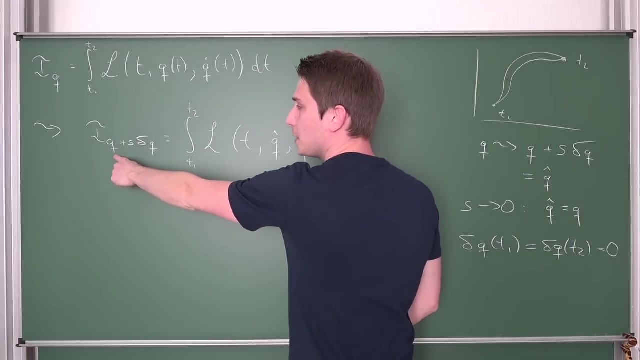 This means that our path is going to be minimized, meaning it's equal to our original path. basically, We would like to differentiate this, but with respect to what? Now we just need to take a look at the variables. if it were dependent on Q or Delta Q, Then this wouldn't make any sense, because we are integrating. with respect to T. 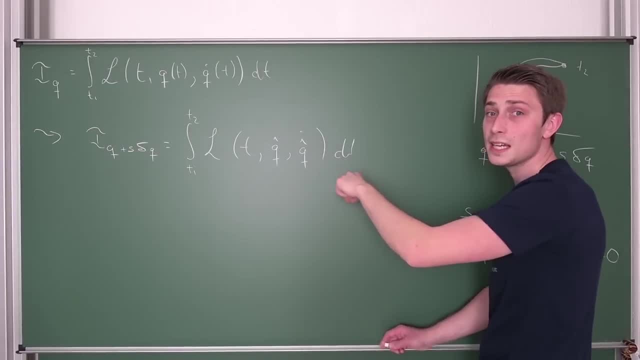 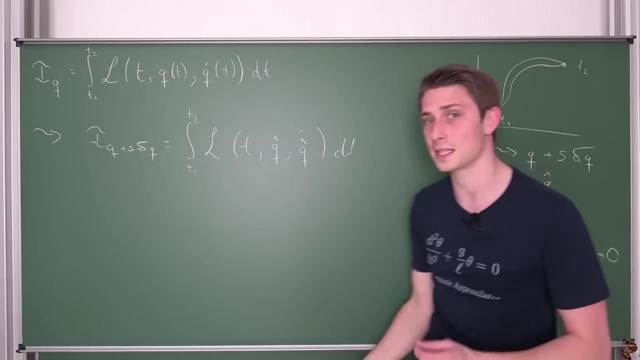 q, het and qhet dot are also functions with respect to T, So integrating those is just going to result in some constants. So the only parameterization that we have in here is with respect to s, meaning we could differentiate this thing with respect to s and see when it's going to be minimized. This also makes sense when 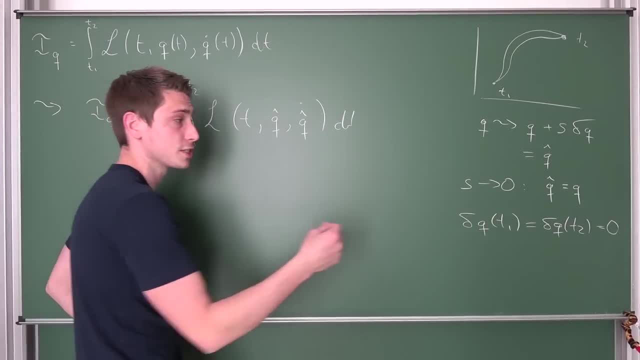 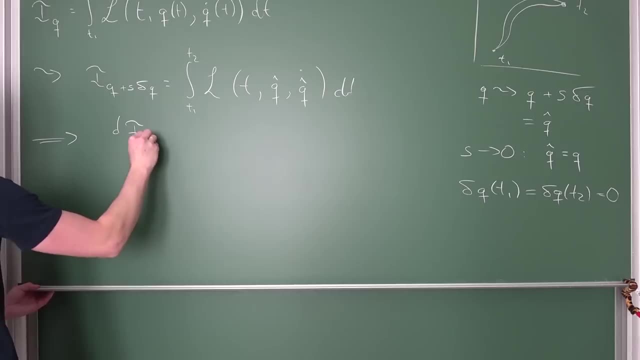 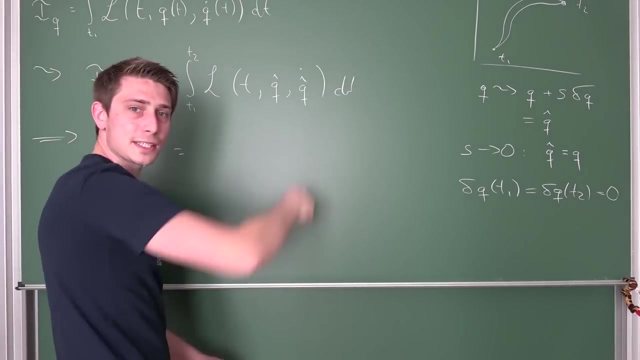 you take a look at this condition: when s goes to zero, our function is going to be minimized. here again, q hat is equal to q, meaning overall, we are going to take d, i, q, q hat. i'm going to call it q hat. ds is equal to well. the differential of this integral, the up and down bounds, are not dependent. 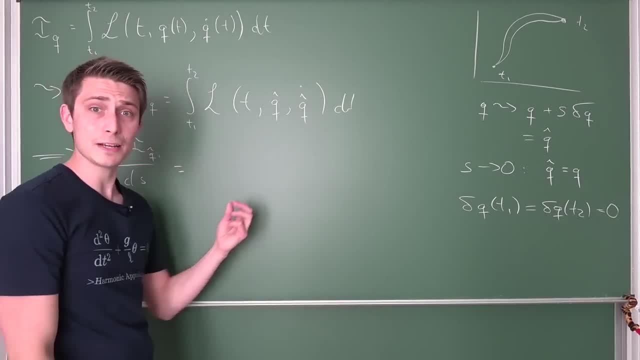 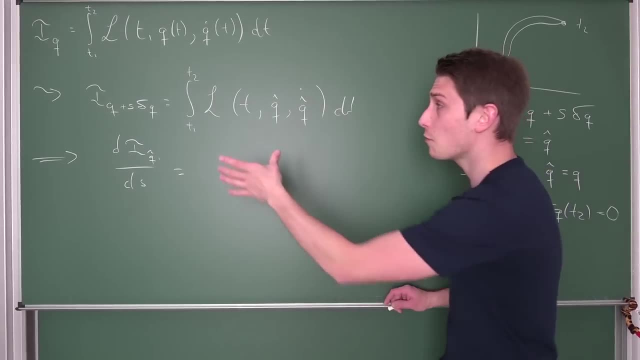 on s here, not dependent on the degree of variation. meaning we can make use of the special case of the leibniz rule. If you don't know what it is, take a look into the description. If our function in here is nice enough, we can actually interchange this limit. so the differential operator and this. 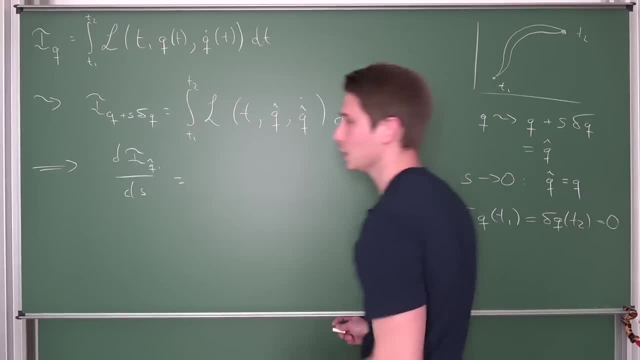 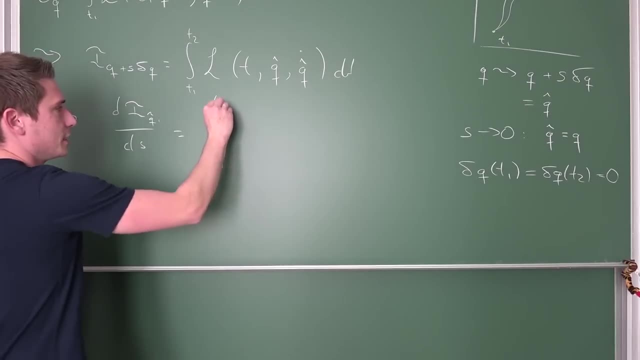 limit our integral and turn it into a partial derivative in here. okay, if you don't know what it is, just take a look at some of my videos, or the explanatory video on the leibniz rule of integration. So this is actually the integral from t1 to t2 of del s, so the partial derivative. 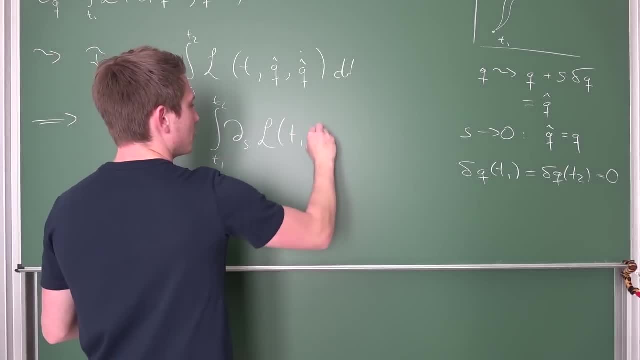 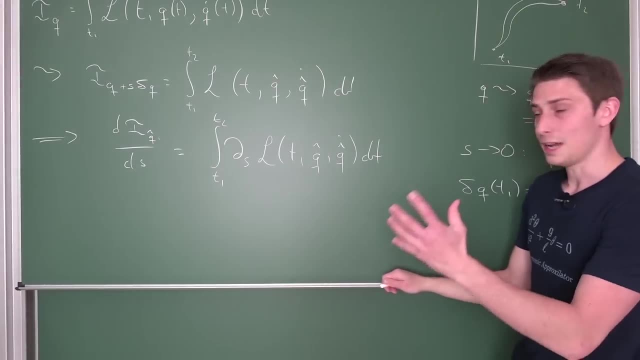 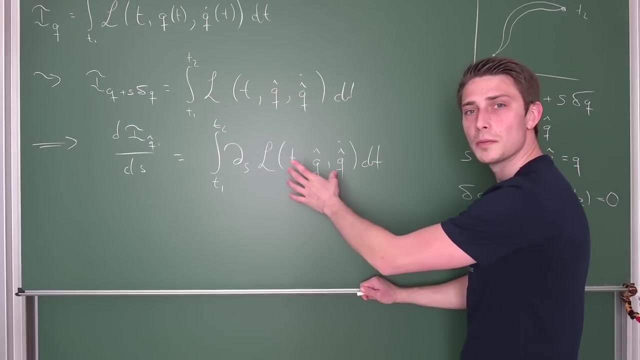 derivative in S of our Lagrangian, that we have t, q hat comma, q hat dot integrated with respect to t And now we can start to differentiate this thing. Now you might ask yourself how could we differentiate a multivariable function? Let us take a look at a function in two variables. 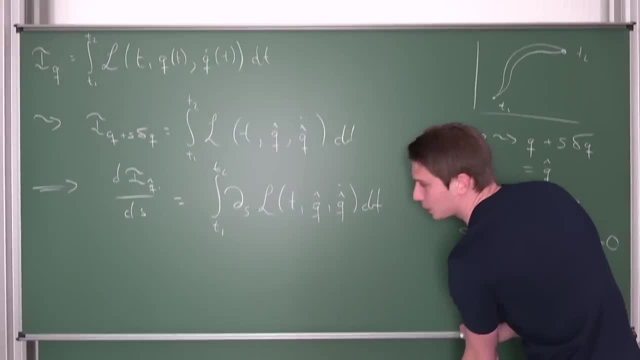 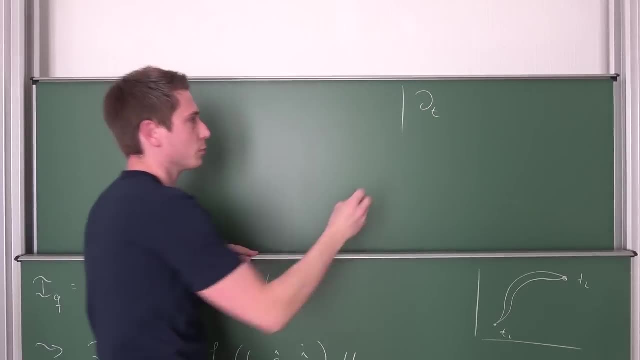 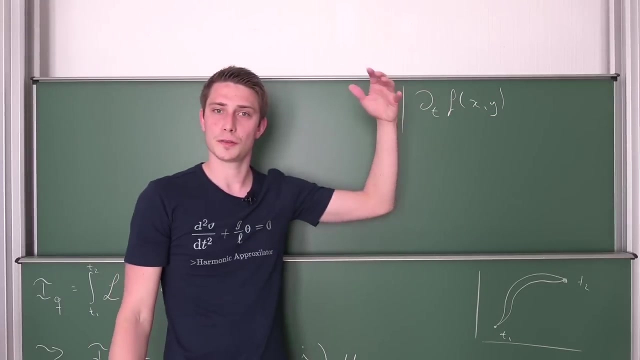 okay, and how we could differentiate it with respect to x, for example. So let us take a look at del t. or we are going to differentiate it with respect to t of f, x, comma y, where x and y are also dependent on t. This is just the chain rule, okay. Maybe you know it in. 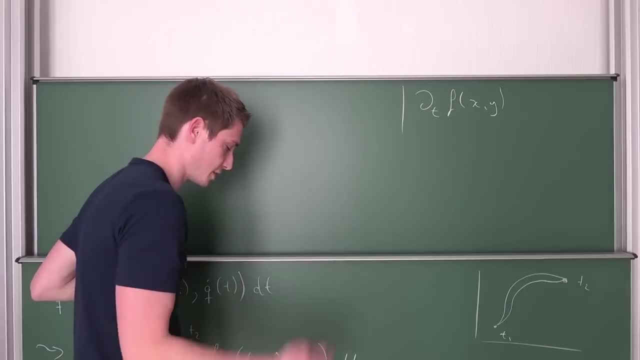 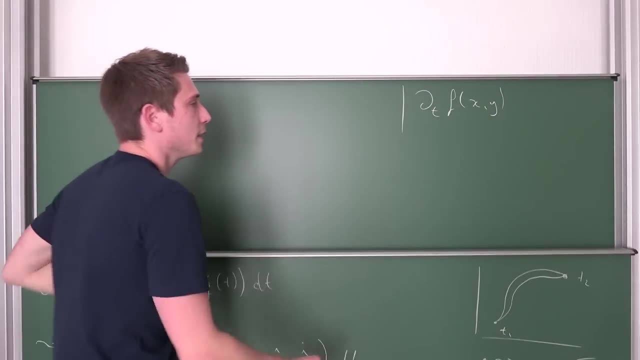 one dimension. There is a generalization for n dimensions. We only need two dimensions here, though, because we only have those two variables, q hat and q hat dot, being dependent on S, actually Meaning overall, if we were to use the chain rule, we are going to end. 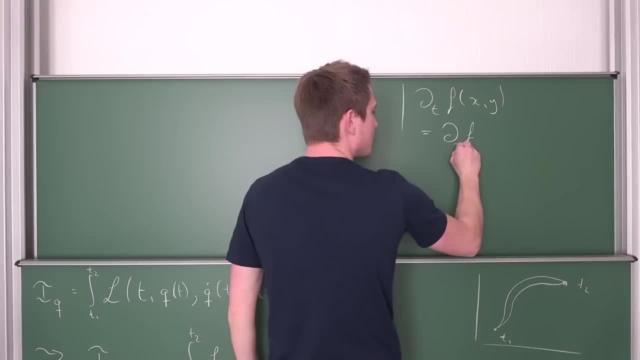 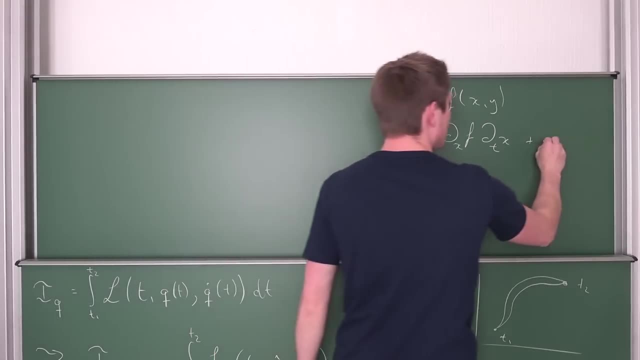 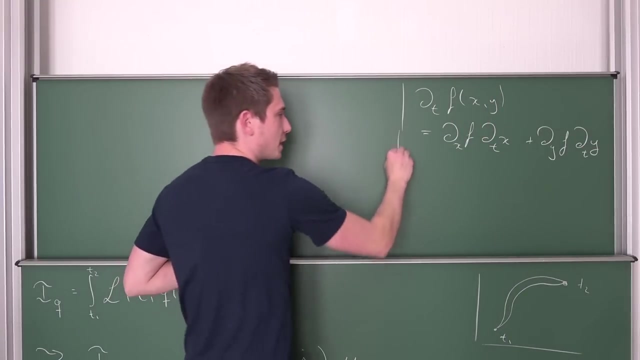 up with the derivative of our f in x times the derivative of x in t, plus the same thing, just with a y substituted into here instead of an x Del y, f del y, t. Now we are going to apply this exact method to our Lagrangian that we have here, Meaning our integral is going to stay. 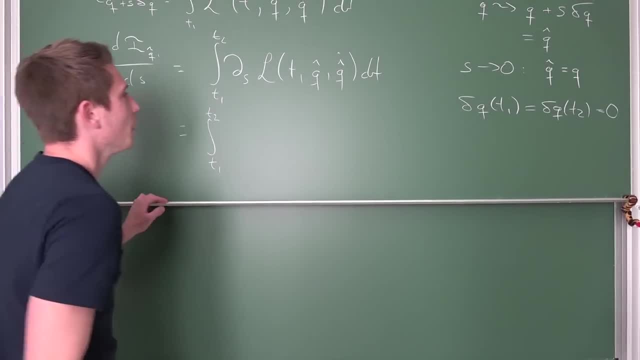 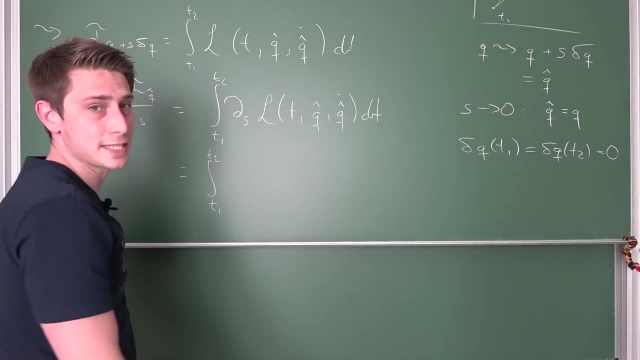 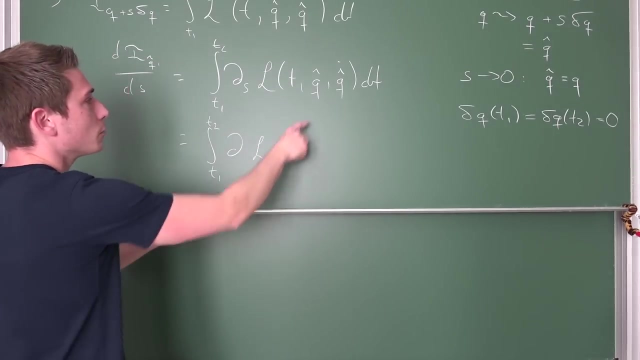 where it is. So the integral from t one to t two of this first variable, in here t, is not dependent on s meaning. we can just throw it out of the window, let it die in Mexico somewhere getting eaten by hyenas. Now we are going to differentiate, at first our Lagrangian with 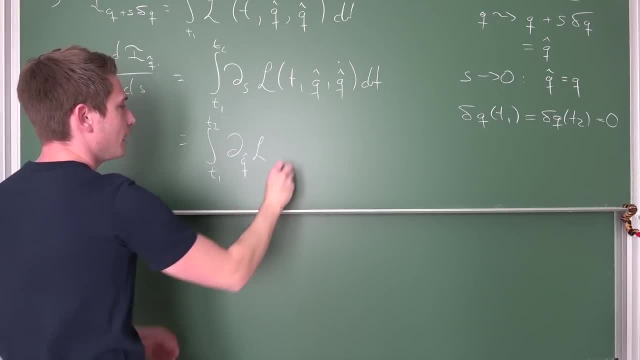 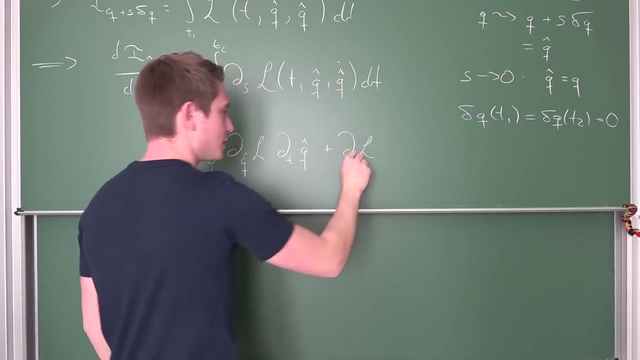 respect to the first variable, q hat, and then we are going to multiply it by the differential of q hat in t. Okay, it's as easy as it is, Plus okay. next up is our differential of the Lagrangian in q hat dot. that's kind of a variable mess that we have right here del q hat dot. 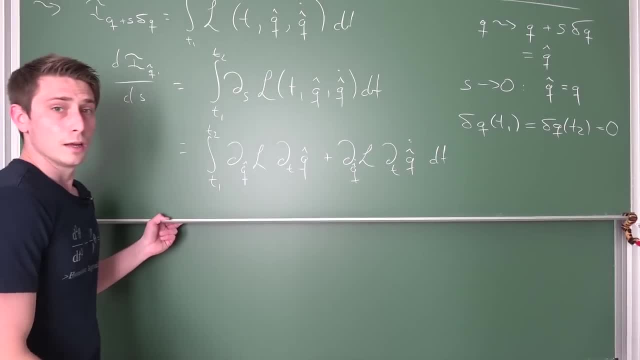 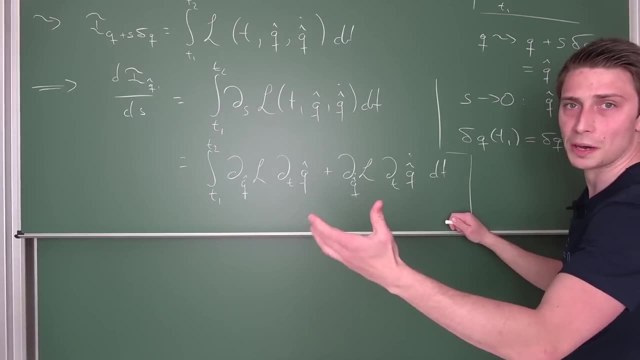 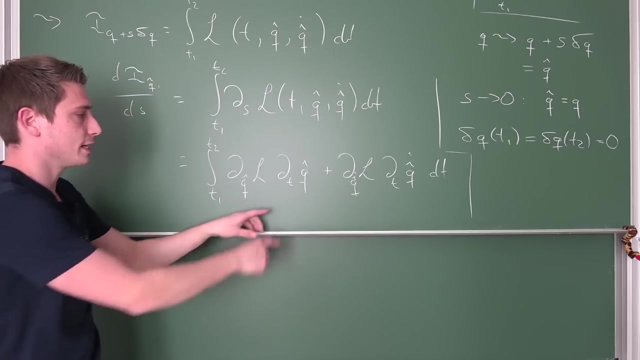 dt. Okay, that's a lot of stuff we had to write out here. it's a lot of thinking we have to do. okay, just bear with me for a minute longer. we are basically already done. Now we can actually simplify some more stuff here if we were to take a look at the differentials of our- oh no, we are. 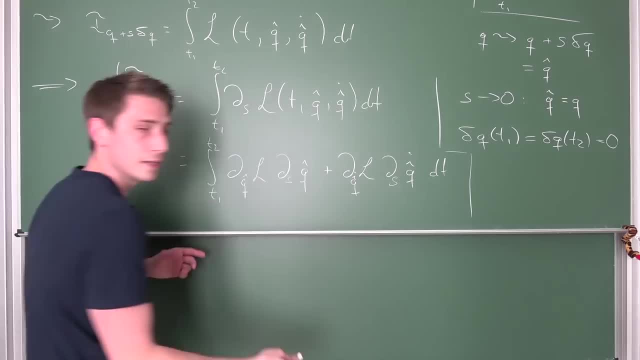 going to differentiate with respect to s here. I'm telling you that we are going to differentiate with respect to s here. I'm telling you that we are going to differentiate with respect to s here. Sorry, totally messed it up. because of the rule that we have right here, mistakes happen. Now we 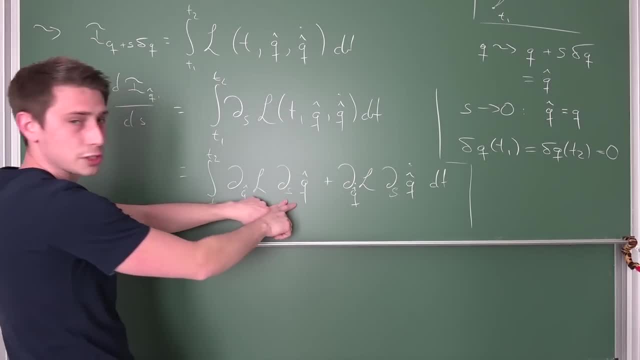 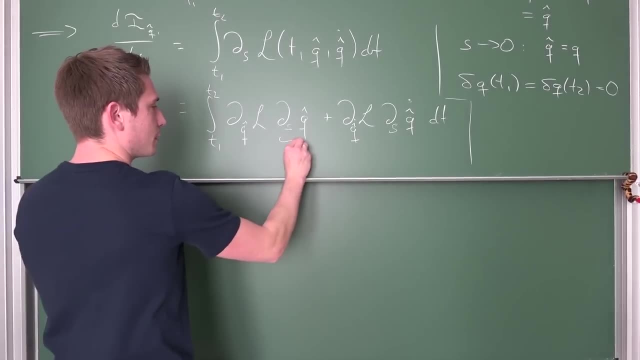 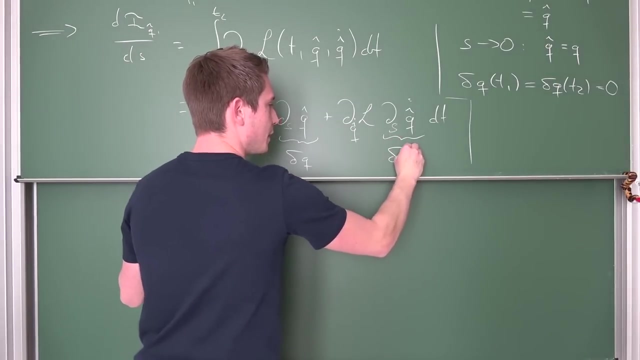 can totally simplify some more stuff here. if we were to differentiate our q hat with respect to s, this means that we are just going to end up with the variation in q here. so delta q. Same spiel goes for this part. we are going to end up with the variation in q, dot. Okay, basically it. 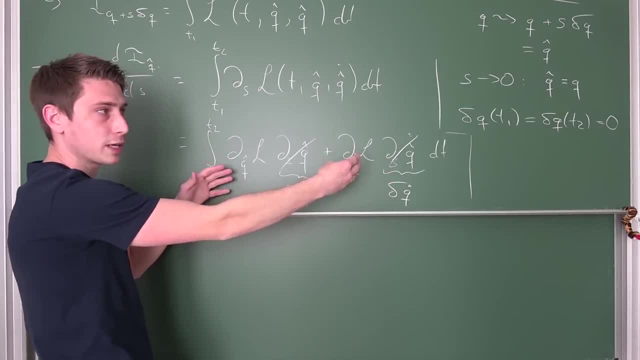 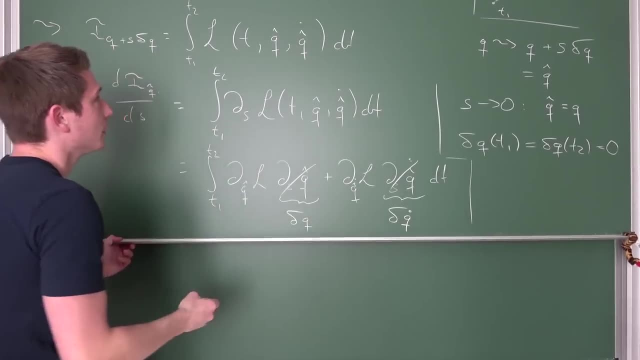 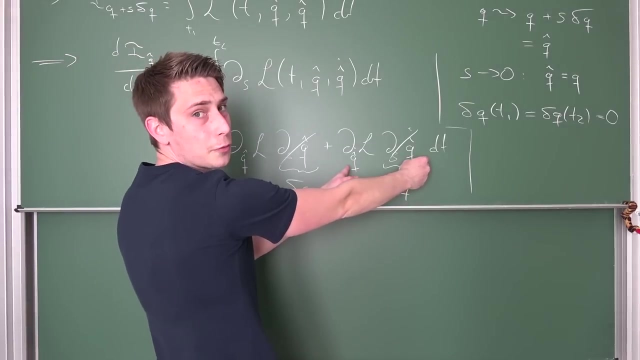 means to kind of evaluate this integral. also, do not forget that we have boundary conditions later that are going to minimize our differential, our function in itself, our i leaving us with the optimized function up here. Now we would like to do some integration by parts on this part, right. 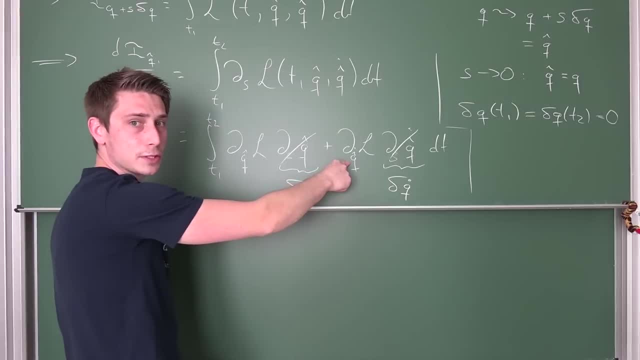 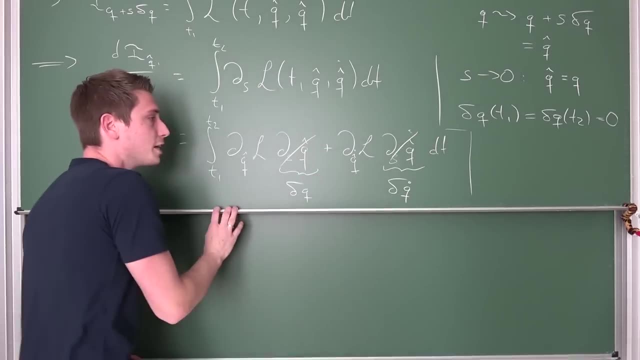 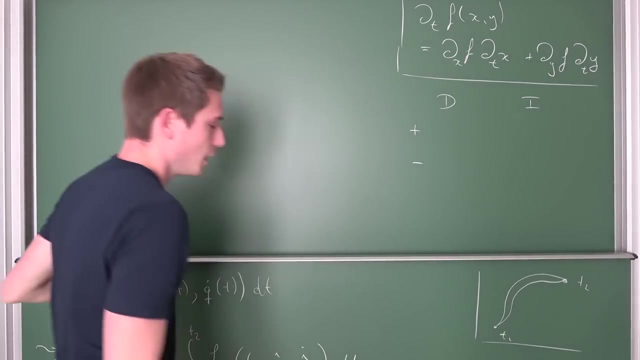 here simply because we are differentiating with respect to a time derivative and we can actually make stuff a bit easier because we are integrating over dt. Okay, so let us just take a look at integration by parts. For this last part, we need something to differentiate and something to integrate. plus minus, What are we? 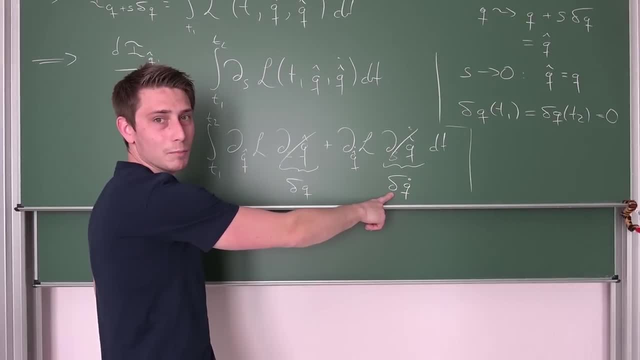 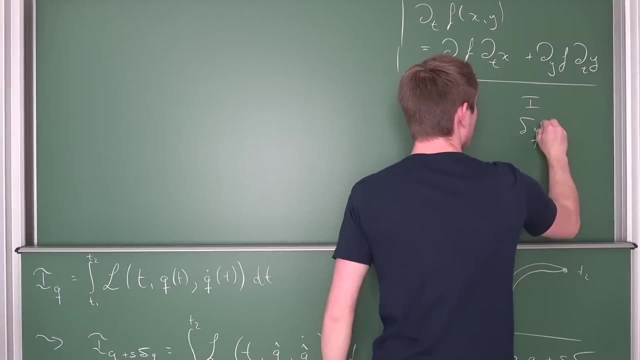 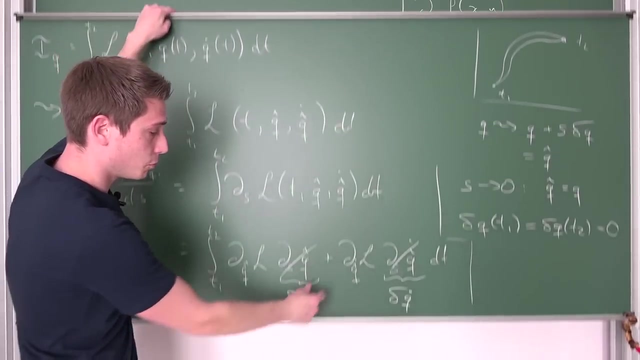 going to integrate. Well, that's the only thing that we can reintegrate, because it leaves us just with the variation in q. Okay, so variation q dot integrated is just a variation in q. Now for the differential. we are just going to differentiate this part. Okay, so this is del q hat dot of the 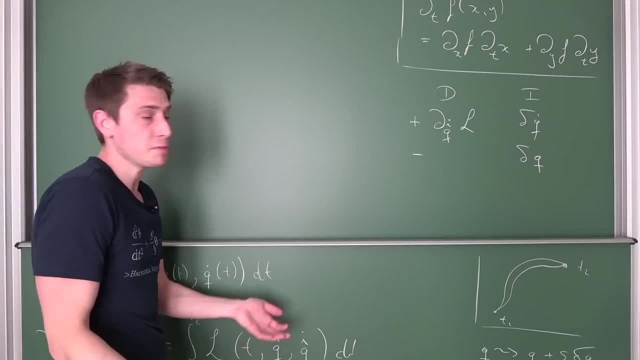 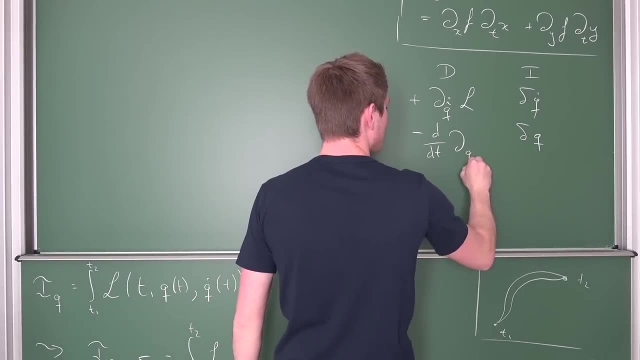 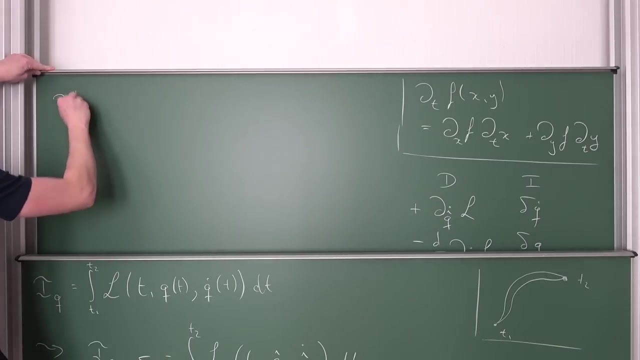 Lagrange, It's nothing but the we don't know, it's a time derivative. if this thing is differentiable, then yeah, let's go ahead and differentiate it. d? dt of del, q, hat, dot of the Lagrange, And now simple integration by parts, meaning overall our i prime. basically, that we are having is nothing but. 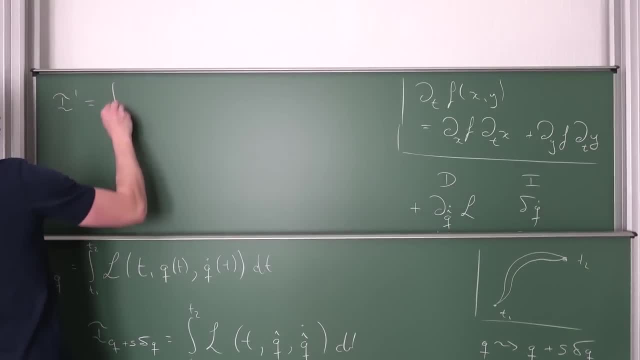 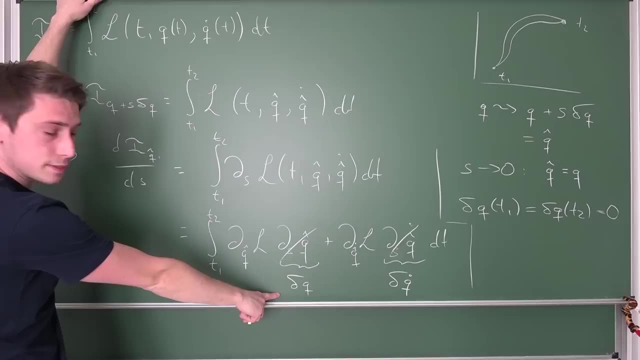 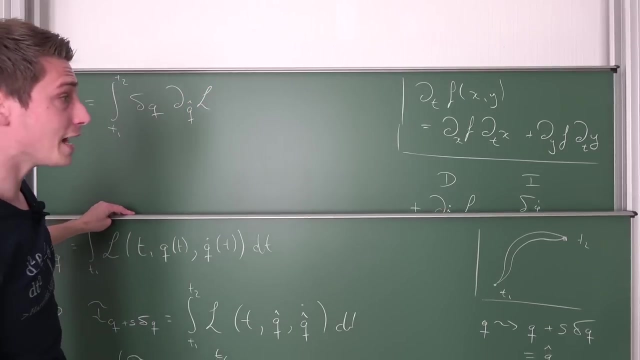 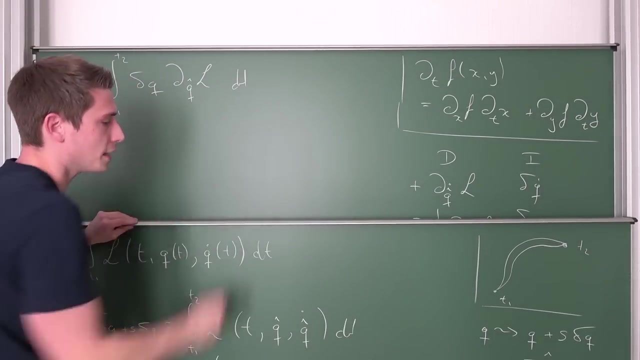 We're going to have this first part here, so that's the integral from t1 to t2 of our variation. This is d dot d dqu times, The differential In q. hat of the Lagrange plus. next up is: This is the part that we are going to do. integration by parts on. 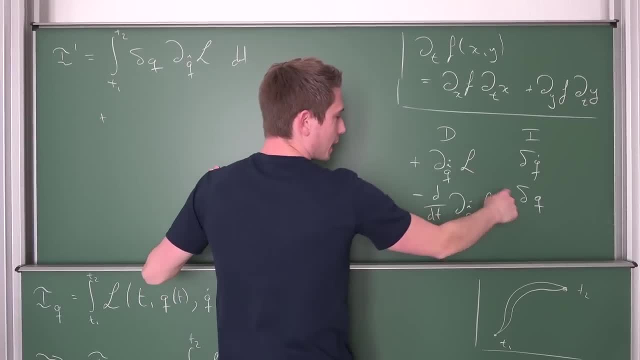 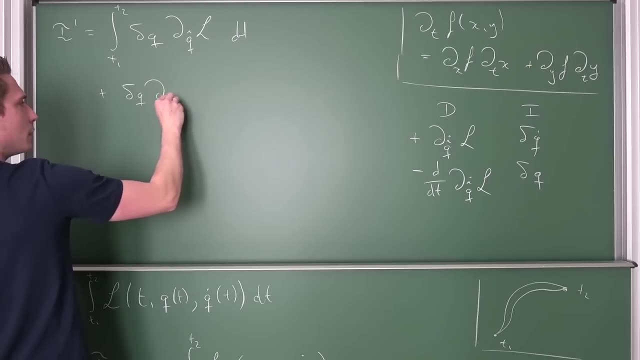 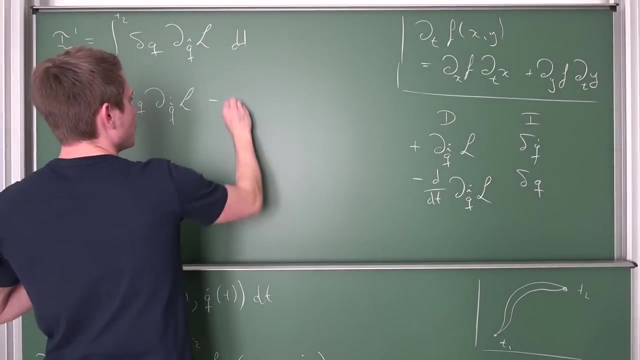 I'm going to close this up Now. integration by parts tells us that we are going to multiply those two together and they getstrom the conditions, meaning we are going to have a variation- times, Q, hat, dot, Lag, subs, Minus those multiplied together, but with an integral around it. Okay, simple integration by parts now. 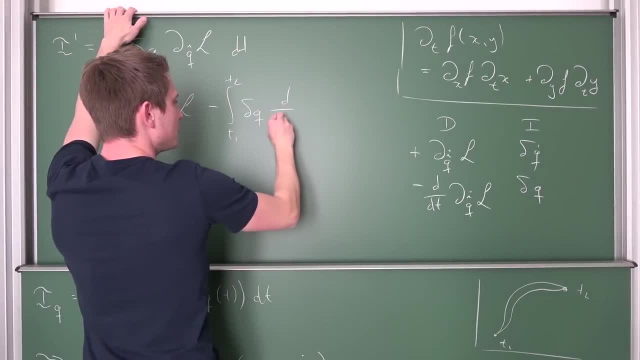 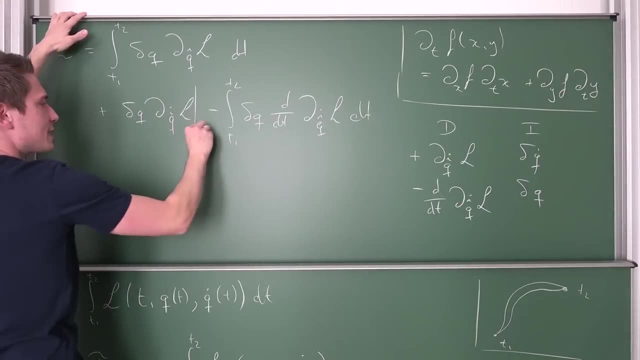 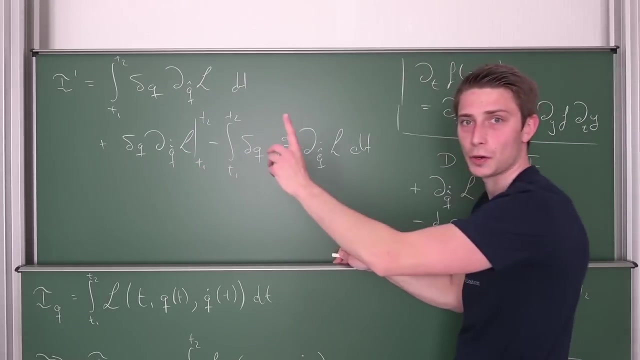 We are going to have our variation in Q, D, D, T, Del, Q, hat, dot, like Russian, integrate with respect to T. Like I said, by applying the boundary conditions We can actually solve this integration by parts problem because if you take a look, our variation vanishes at. 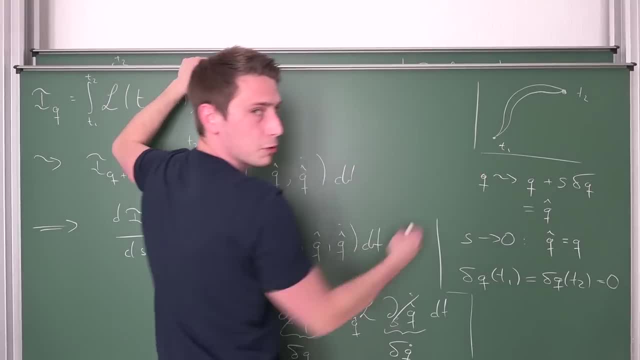 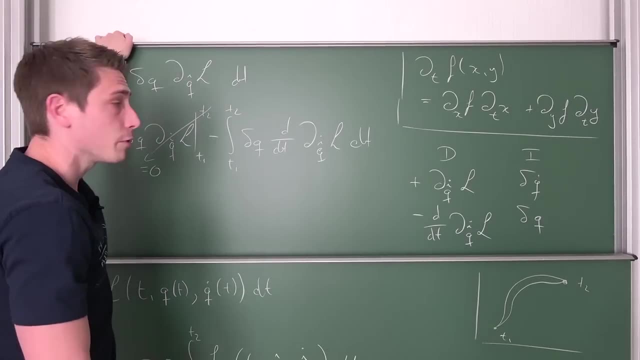 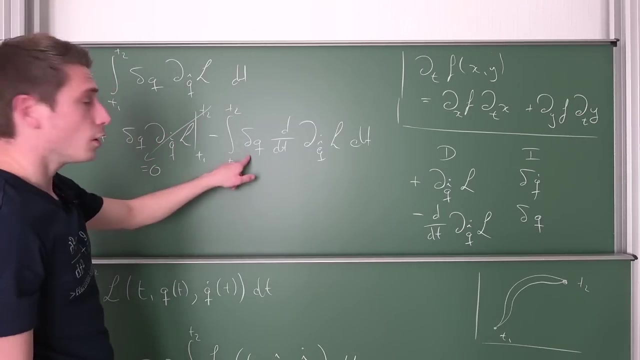 Nodes. this is what we have seen before, because it becomes arbitrarily close to our original curve, Meaning: overall, both parts are zero. This is going to vanish. We are going to make use of the linearity of the integral to bring those two together. Okay, just adding the integrals together into one integral. Also, We have the very same variation here as a common factor, meaning overall, I 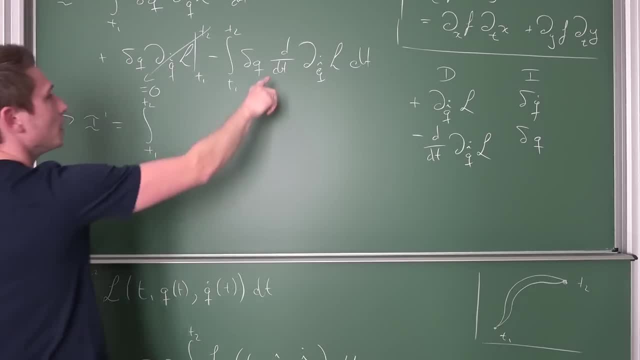 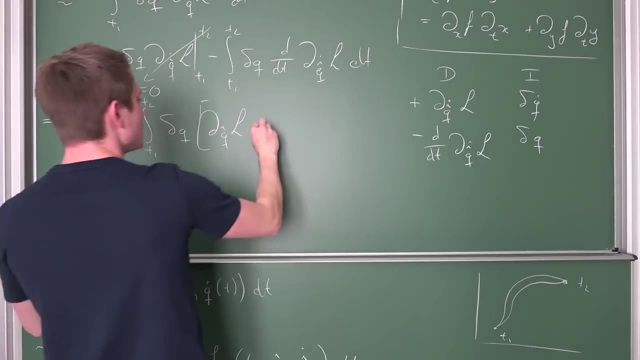 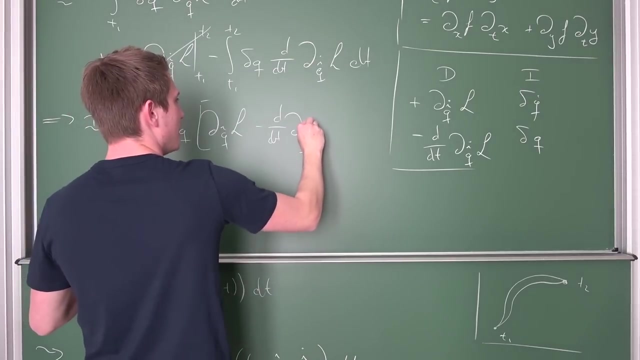 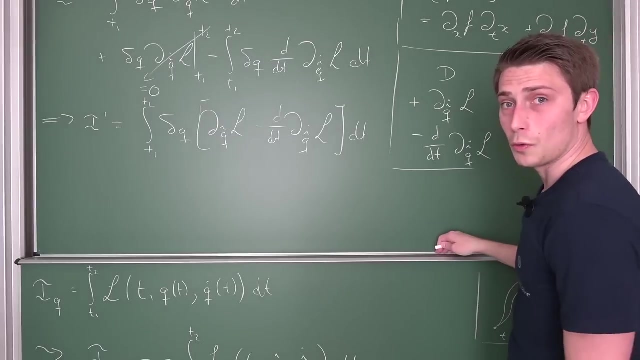 prime is thus the integral from T 1 to T 2 of variation in Q, and then del Q hat, like Russian, minus DDT. I'm going to close this off. DDT, del Q hat, dot, like Russian, integrate with respect to T. one last thing: We are seeking a minimization of this function here. Do not forget when this is going to happen. 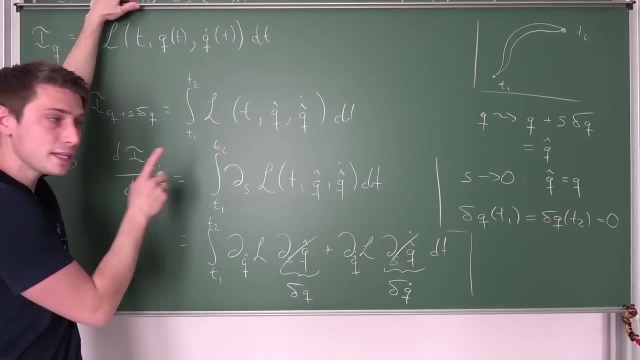 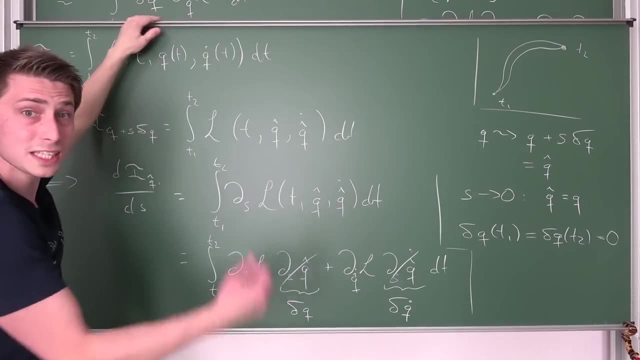 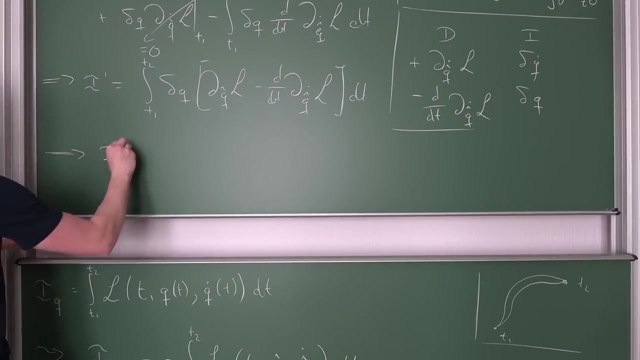 Exactly when we differentiate this and this is equal to zero. when it's going to be Equal to zero is exactly when we apply our boundary condition here s going to zero. This is when we are going to minimize our function, exactly meaning overall- I Prime at s. being equal to zero is nothing but zero. 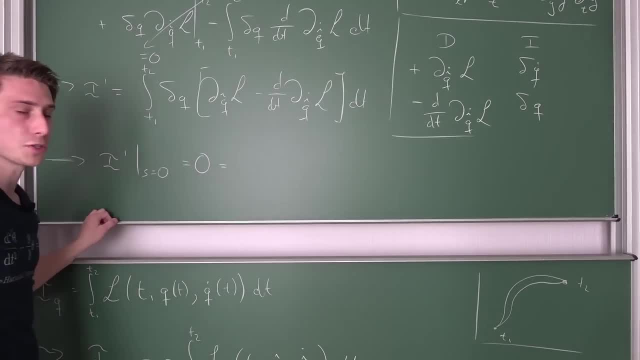 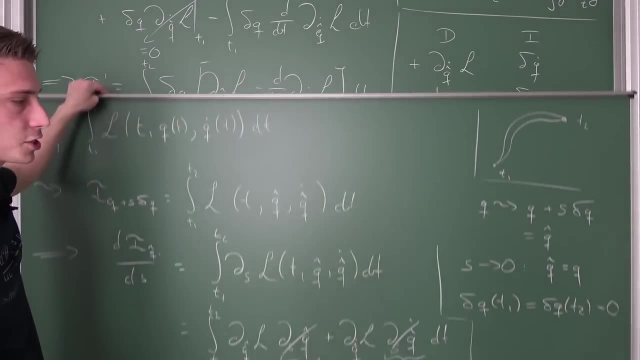 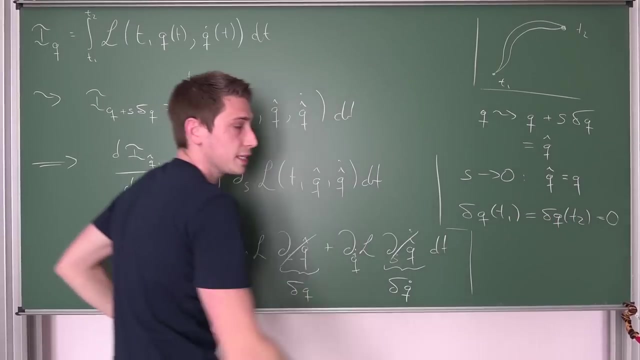 We are going to plug s being equal to zero into here. Also, this part is not going to change overall, But here on Q head and Q head dot, something is going to change. if we let s go to zero, This is just going to be Q and Q dot. This is just what we were seeking. 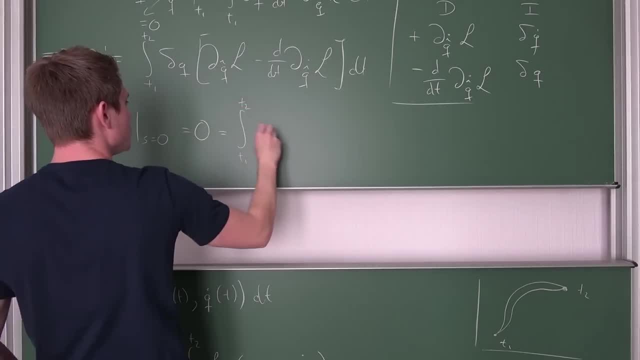 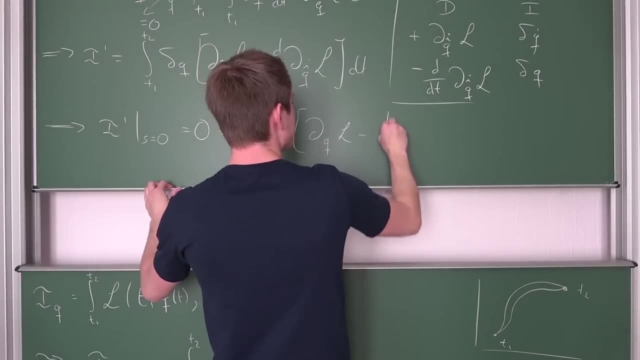 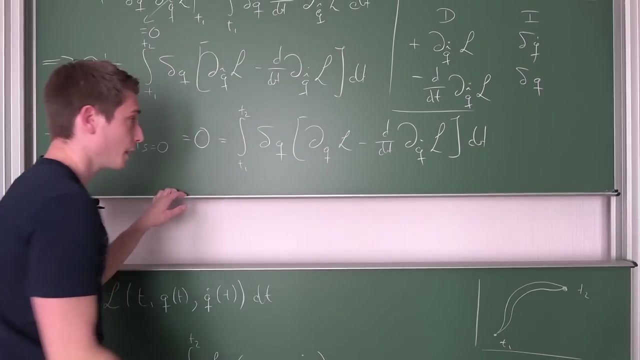 Meaning overall, this is the integral from T 1 to T 2 of our variation times: del Q, like Russian, minus D. DT del Q dot, like Russian, Integrate with respect to T. and here's one last thing: When is a definite integral equal to zero? exactly when. 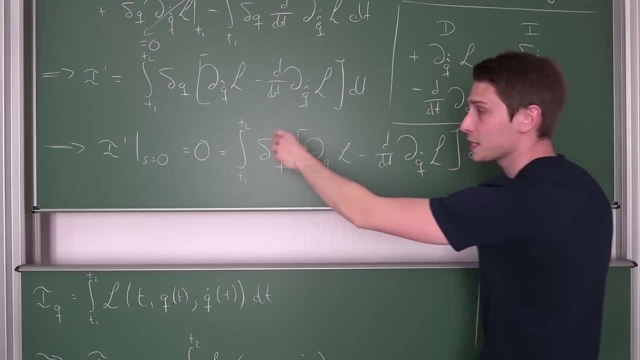 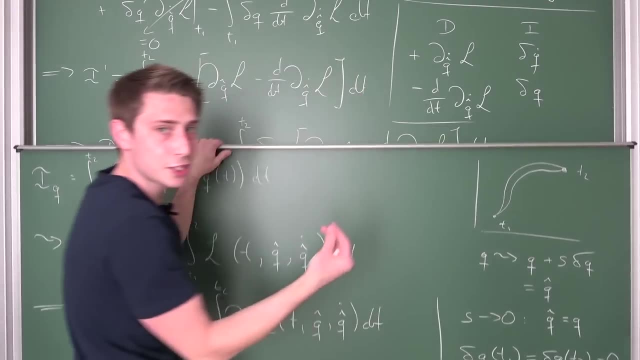 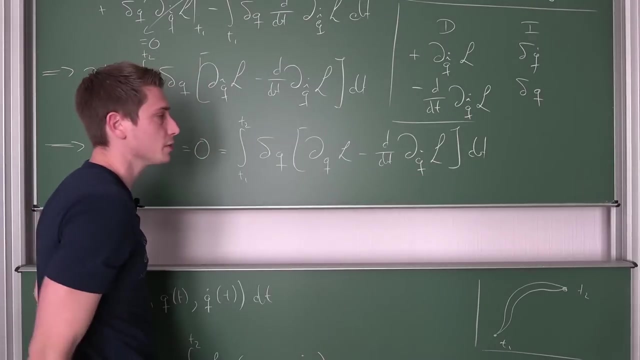 The argument is equal to zero. the argument is multiplication of two things. We don't want our variation to be equal to zero. Okay, it's just something that does stretch our function in some way. We don't want it to be equal to zero. This is what I said at the beginning, meaning overall, in order for this product to be equal to zero.